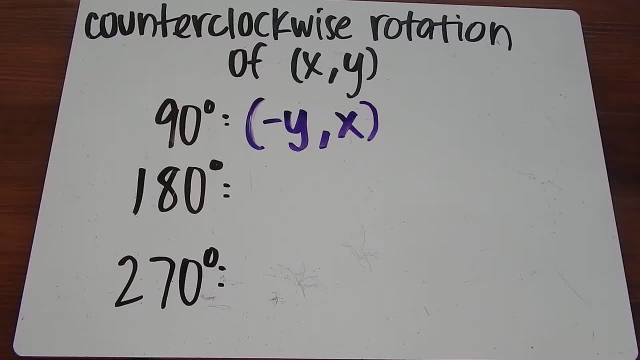 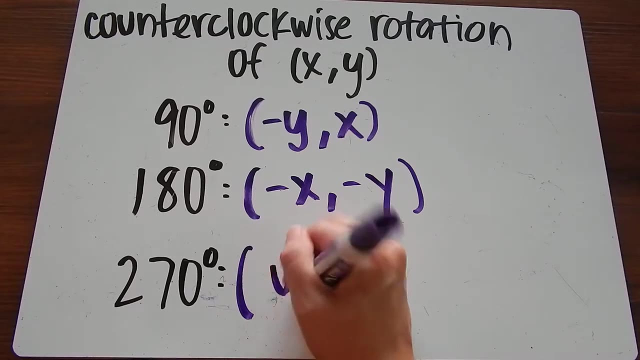 When we rotate that same point 180 degrees, our new point is going to be negative x, negative y. And when we rotate that point 270 degrees, our new point is going to be negative y, negative y, And our new point is going to be y, negative x. 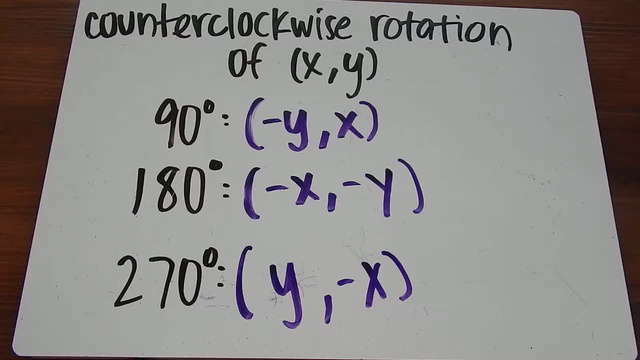 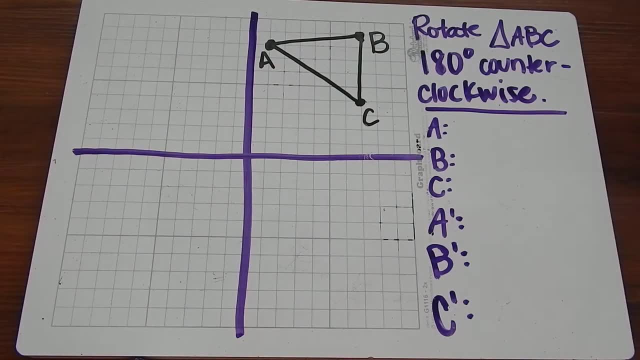 So we will keep these in mind as we go through the examples. So our first example is to rotate triangle ABC 180 degrees counterclockwise. So 180 degrees counterclockwise would be this way: If we're going 180 degrees, that means we need to move two quadrants. 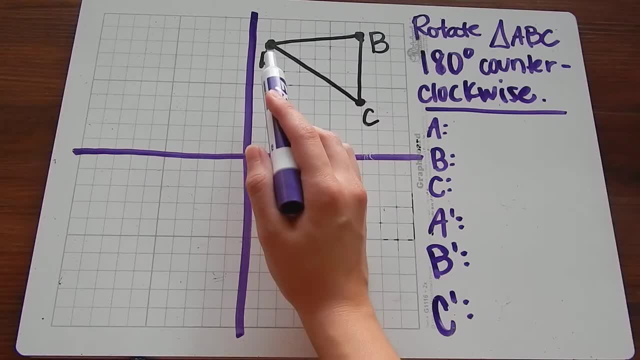 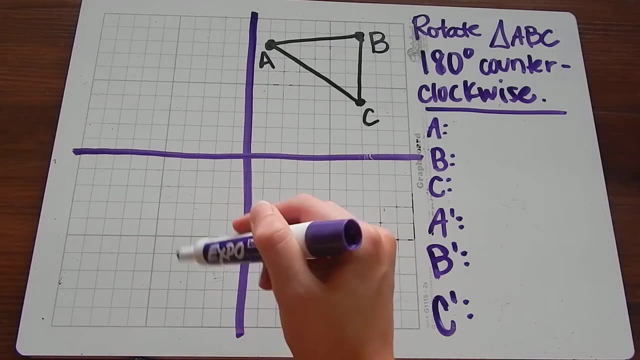 Because each quadrant is 90 degrees. So our new triangle is going to be here two quadrants over. So if we don't get points in this quadrant, we know we did something wrong. The first thing I want to do is label or list my points A, B and C, the coordinates of my points. 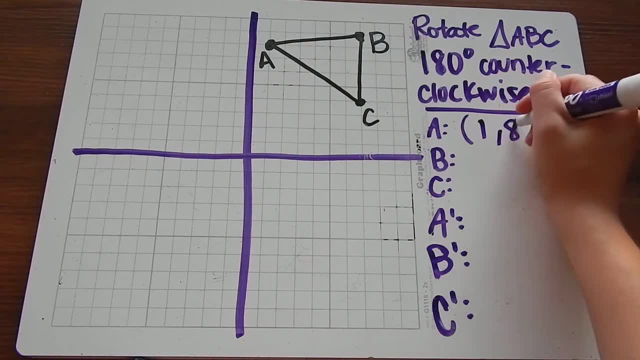 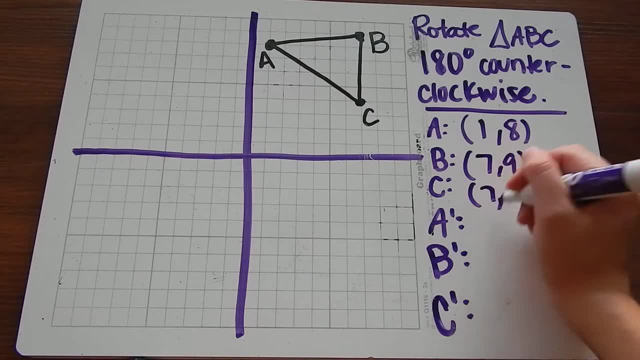 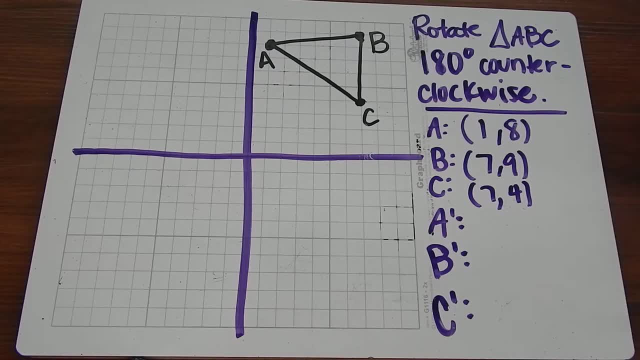 And then we can actually put them on our coordinate grid. So for 180 degrees counterclockwise, our new point is going to be negative X, negative Y. So we're just taking the X and the Y and making them negative. So my A prime is going to be negative 1, negative 8.. 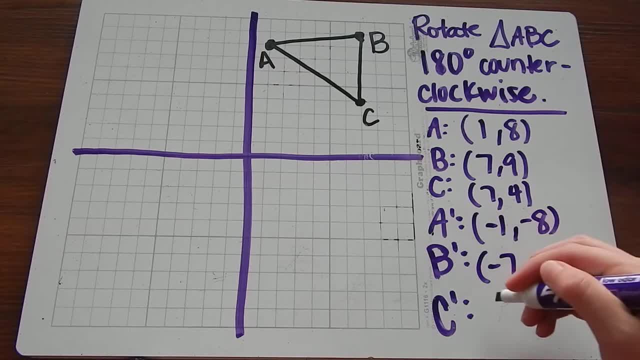 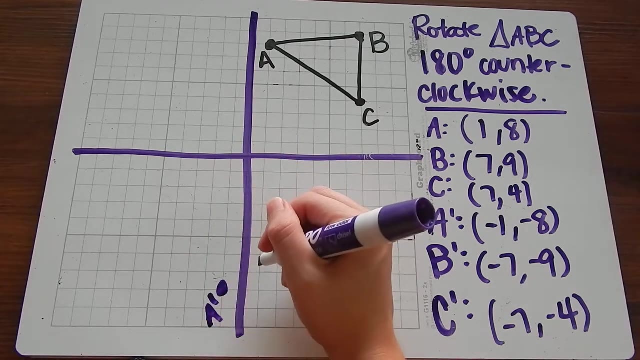 B prime is negative, 7, negative 9.. C prime is negative 7, negative 4.. And we can actually plot those points and draw our new triangle. So A prime is negative, 1, negative 8.. B prime is negative, 7, negative 9.. 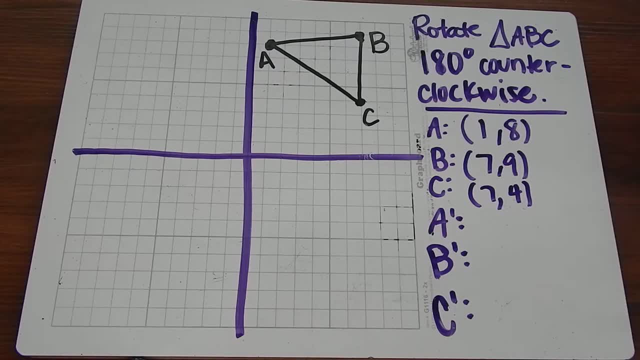 And then we can actually put them on our coordinate grid. So for 180 degrees counterclockwise, our new point is going to be negative x, negative y. So we're just taking the x and the y and making them negative. So my A prime is going to be negative 1, negative 8.. 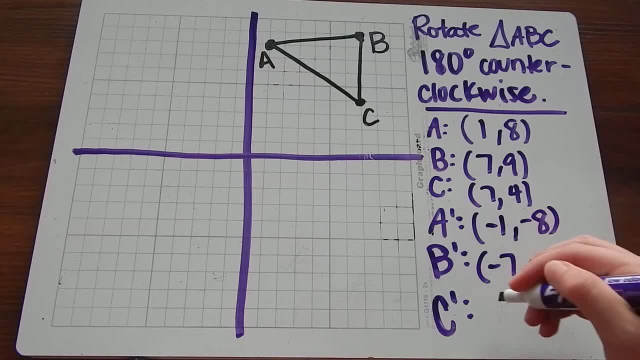 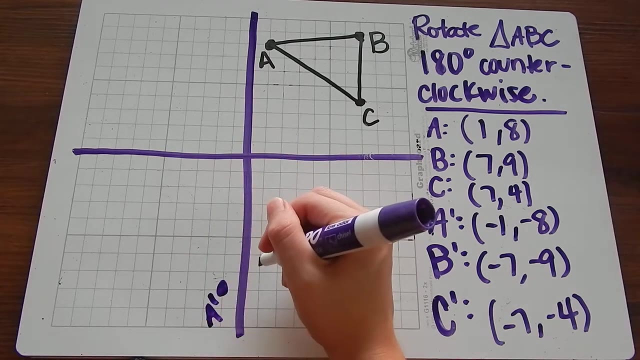 B prime is negative, 7, negative 9.. C prime is negative 7, negative 4.. And we can actually plot those points and draw our new triangle. So A prime is negative, 1, negative 8.. B prime is negative, 7, negative 9.. 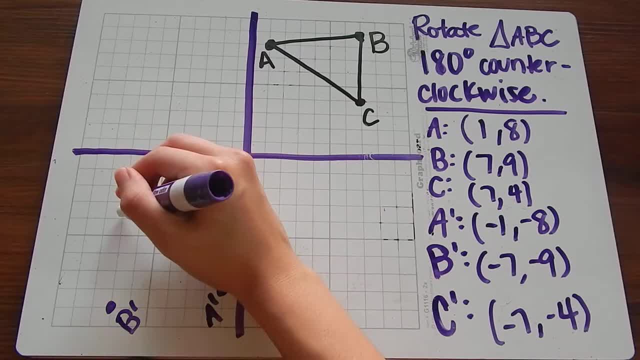 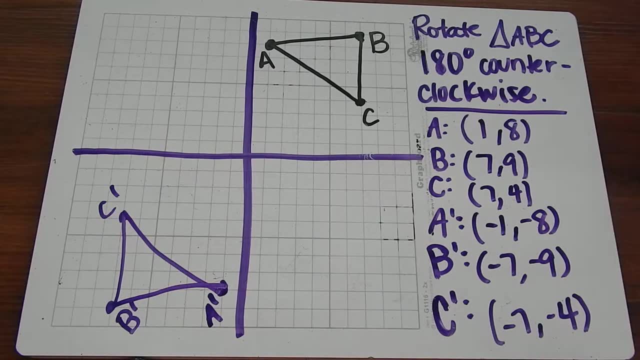 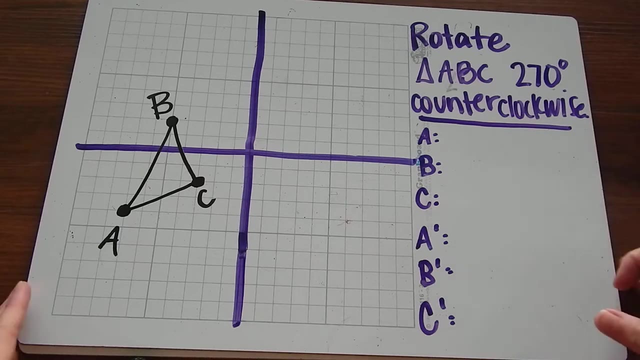 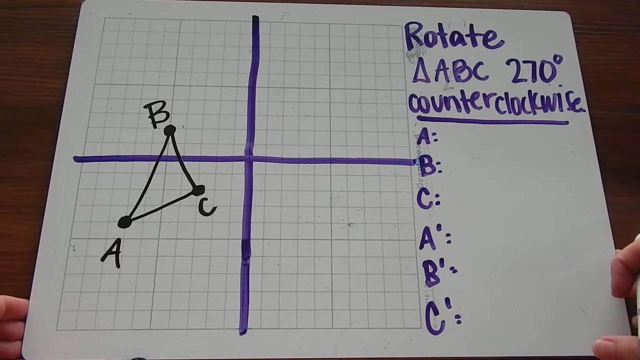 And C prime is negative 7.. And C prime is negative 7, negative, 4.. And here is our new triangle. Our next example says rotate triangle ABC, 270 degrees, counterclockwise. Again, we're going to start by listing the coordinates. 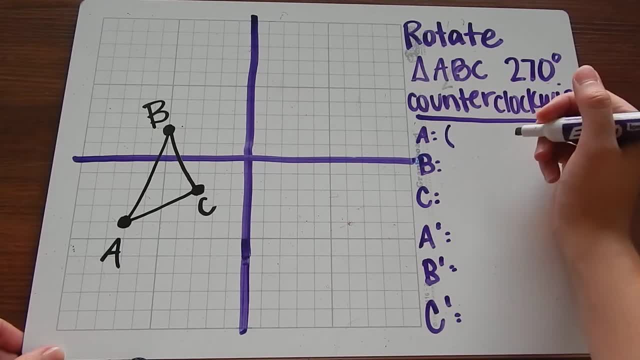 So coordinate for point A. Point A is going to be negative 7, negative 4.. Point B is negative 5, 2.. Point C is negative 3, negative 2.. When we rotate counterclockwise 270 degrees, we need to move three quadrants. 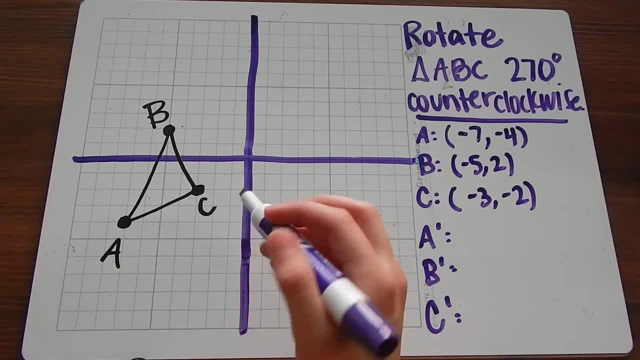 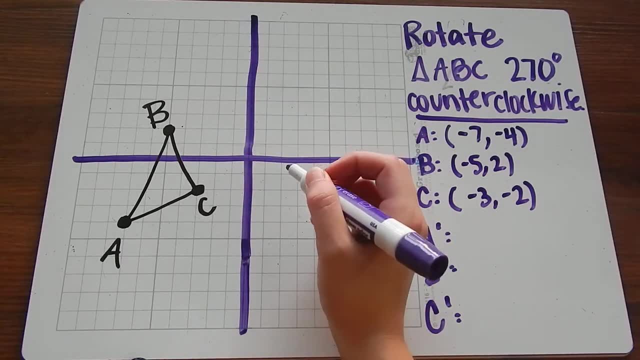 Three, because 270 divided by 90 is 3.. Each quadrant is 90 degrees, So each point needs to be three quadrants away, counterclockwise, from where it was. So A and C are going to end up here. B is going to end up somewhere here. 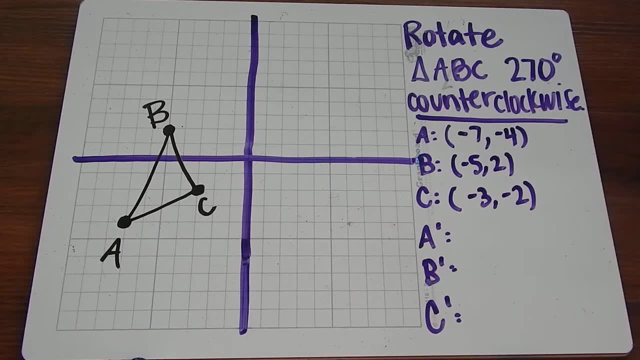 Make sure you're checking for that as you write your new points and plot them. So our rule for rotating 270 degrees is y negative x. So we're going to keep the y. Now it goes First the x. we're going to change the sign and that's our new y. 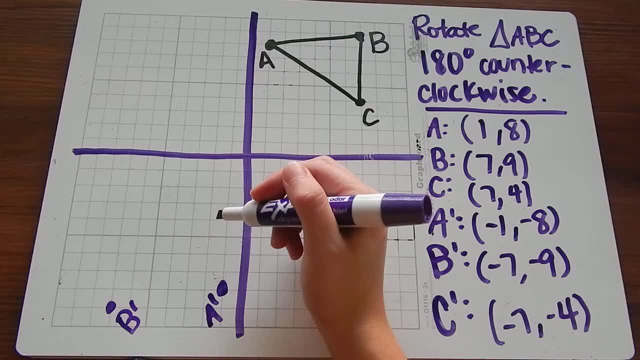 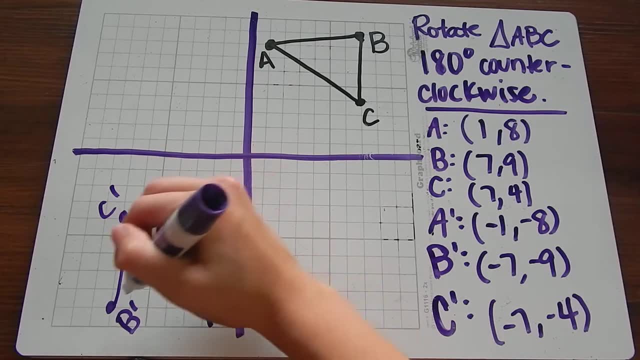 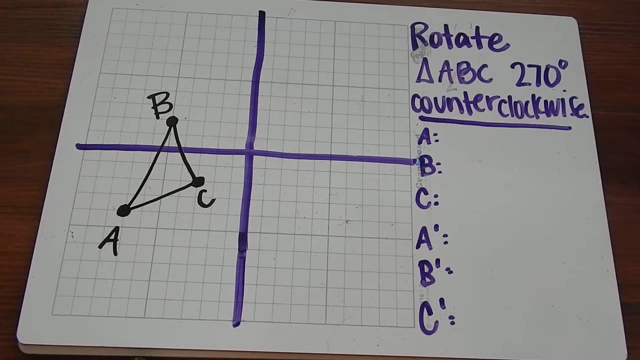 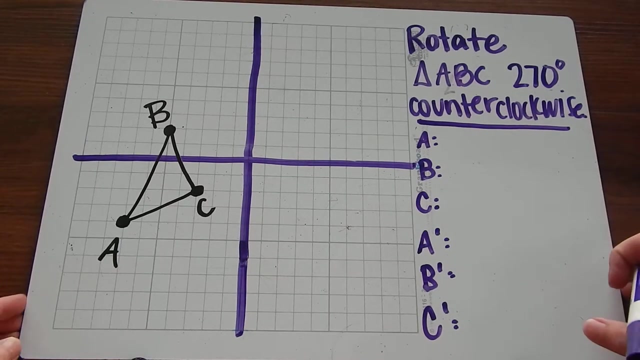 And C prime is negative 7.. And C prime is negative 7, negative, 4.. And here is our new triangle. Our next example says rotate triangle ABC, 270 degrees, counterclockwise. Again, we're going to start by listing the coordinates. 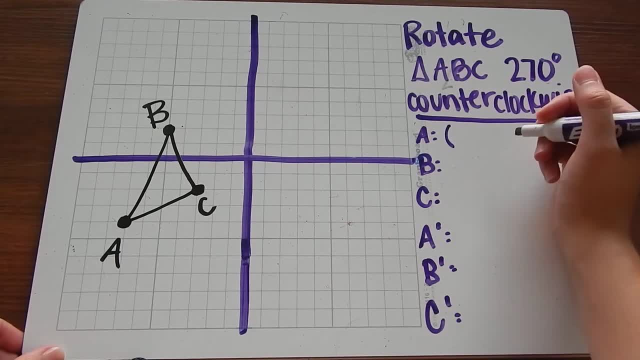 So coordinate for point A. Point A is going to be negative 7, negative 4.. Point B is 5, negative, 5, 2. And point C is negative, 3, negative, 2.. When we rotate counterclockwise 270 degrees, we need to move 3 quadrants. 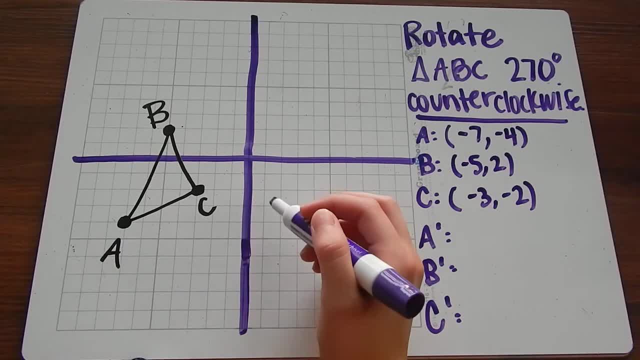 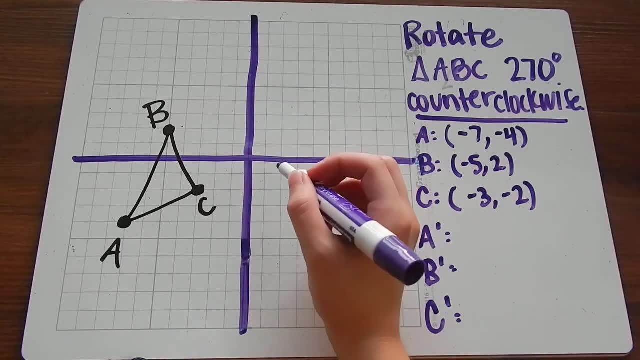 3, because 270 divided by 90 is 3.. So each quadrant is 90 degrees. So each point needs to be 3 quadrants away, counterclockwise, from where it was. So A and C are going to end up here. 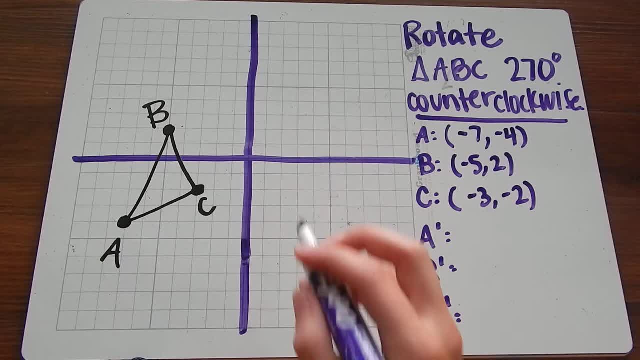 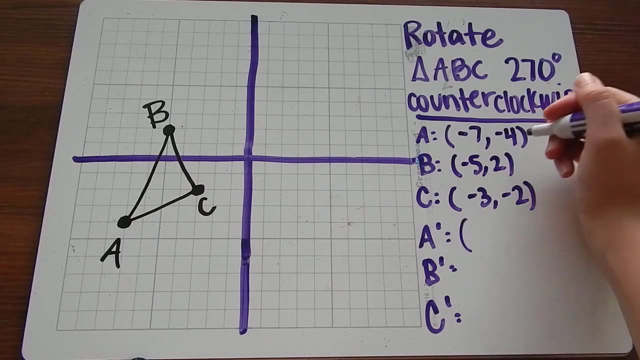 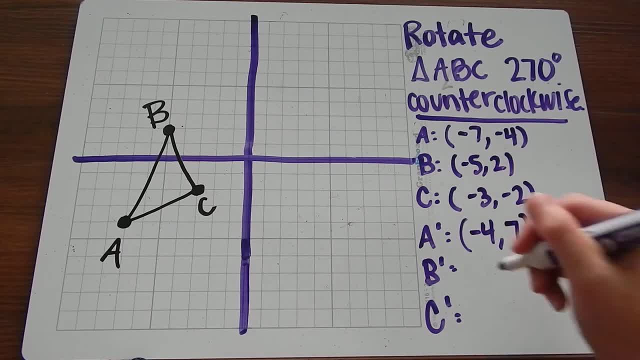 The X. we're going to change the sign and that's our new Y. So again, Y negative X And Y negative 2, negative X would be positive 3.. So we change the signs of the X values. 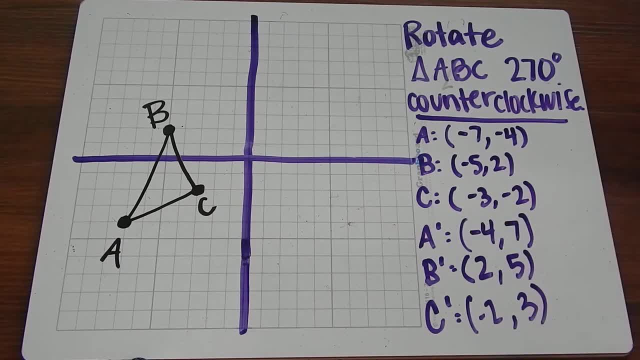 They go in Y, All the Ys stay the same, but they now go in X, And now we can plot these points and draw our new triangle. So A prime is negative 4, 7.. So over here we have negative 4, 7..